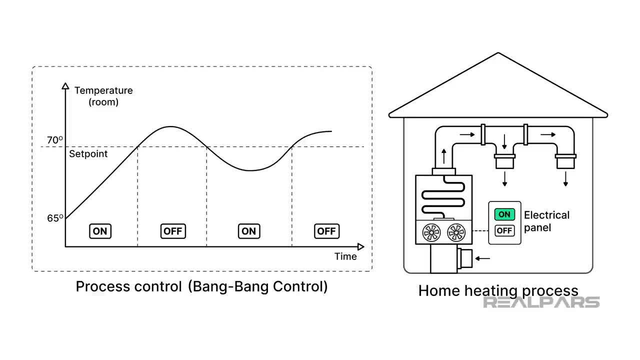 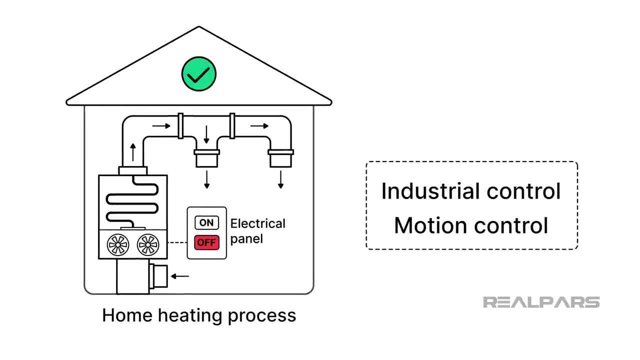 This technique is very common and found in applications such as home heating, where furnace is either on or off. What we end up with is a continuous temperature fluctuation around the desired set point. On-Off control may be okay for a house, but it's not okay for industrial processes. 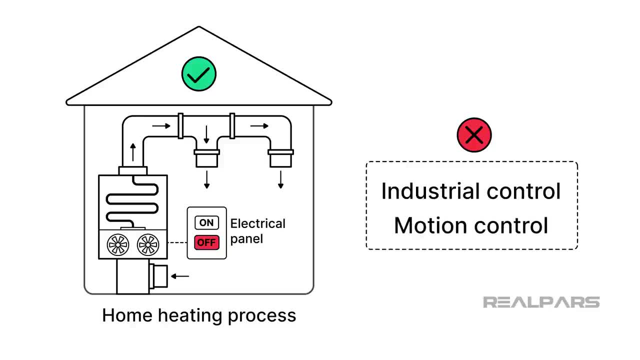 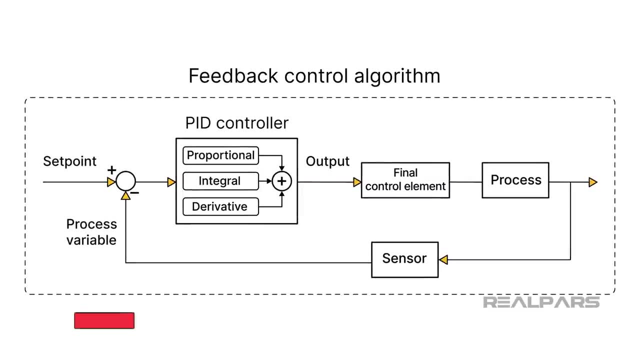 or motion control, as these fluctuations around the set point are not acceptable. Next up on the list is a feedback control algorithm called PID control. The three main components are Proportional, Integral and Derivative. PID control is very versatile and goes a long way to ensure that the actual process 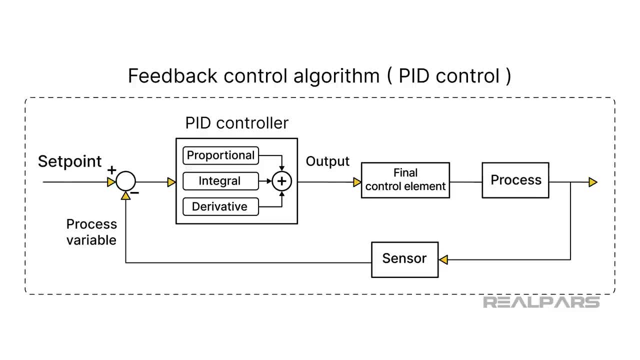 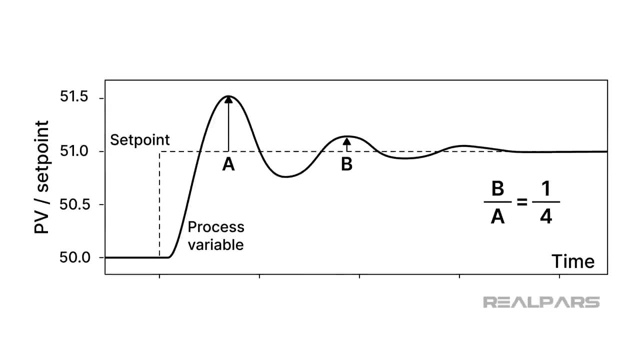 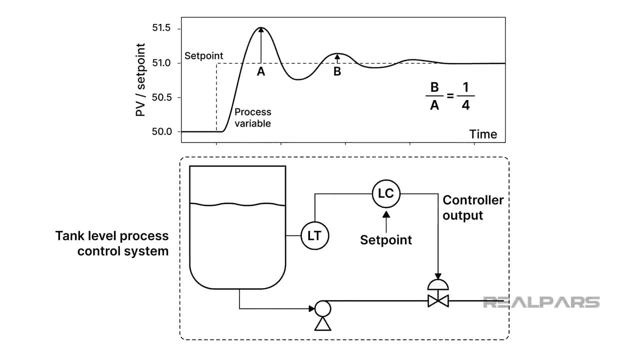 under control is held as closely as possible to the set point, regardless of disturbances or set point changes. For example, PID control produces an acceptable quarter wave response to a 1% set point change in a tank level process control system. However, that quarter wave type of response 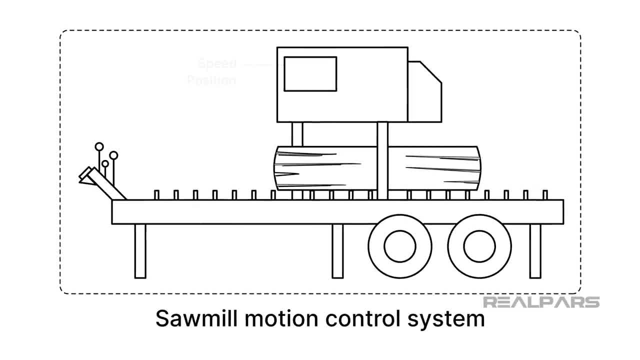 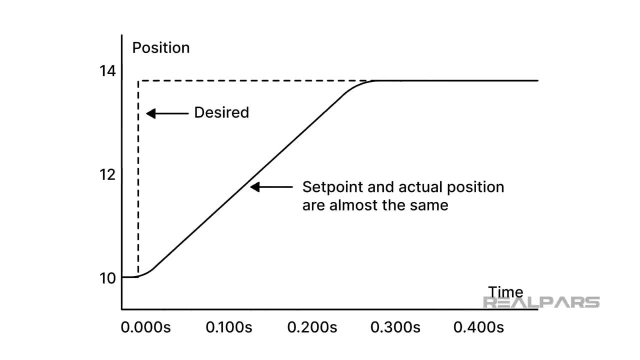 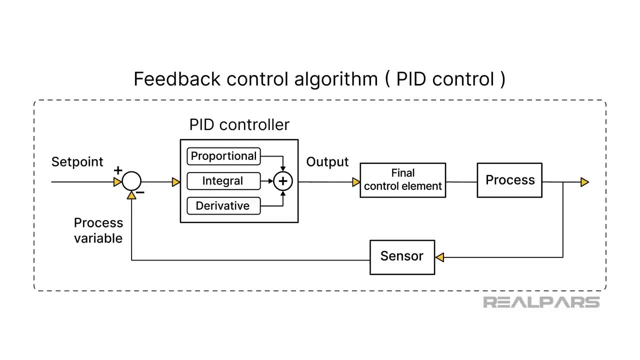 just won't work. in a sawmill motion control system where the speed and position of an electro-hydraulic valve are critical, The valve position cannot be allowed to swing wildly around the set point. Controller tuning involves a procedure where each component of the PID algorithm 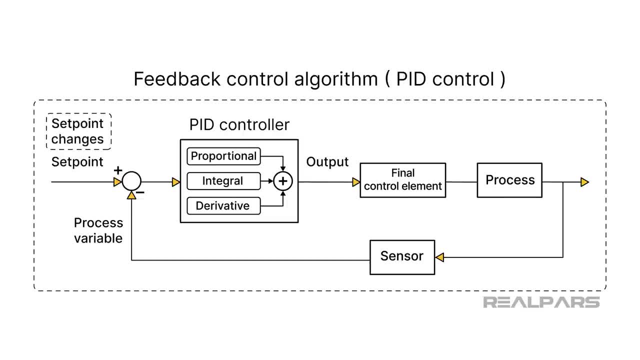 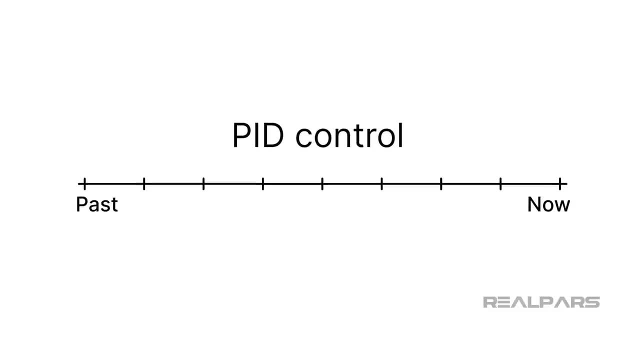 is adjusted to produce the desired response to set point, changes or disturbances. Why is PID control so popular? Well, PID control has been around for a very long time. PID control is taught to engineers and technicians in every college and university. PLCs and DCSs have built-in PID functionality. 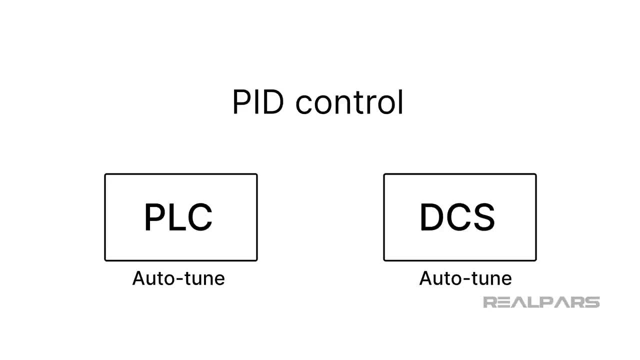 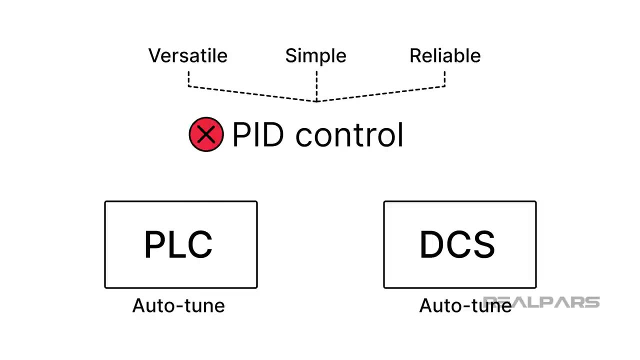 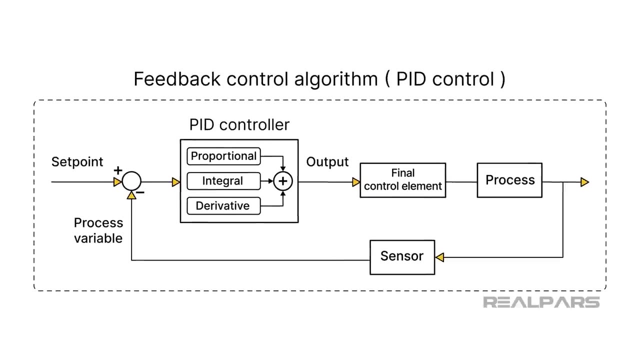 and many have auto-tune features. PID control is simple, versatile and reliable, But it's not always the best choice and many applications are better suited to more advanced control techniques. Alright, let's have a brief discussion on the components of PID control. 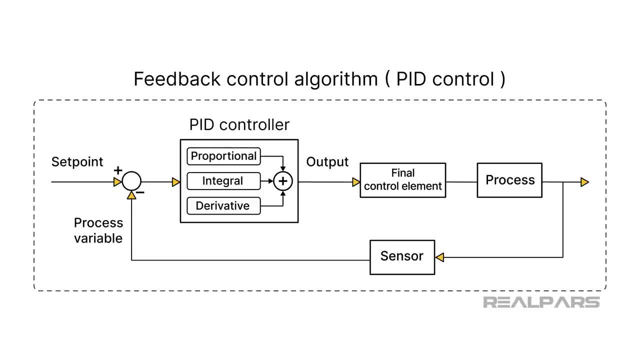 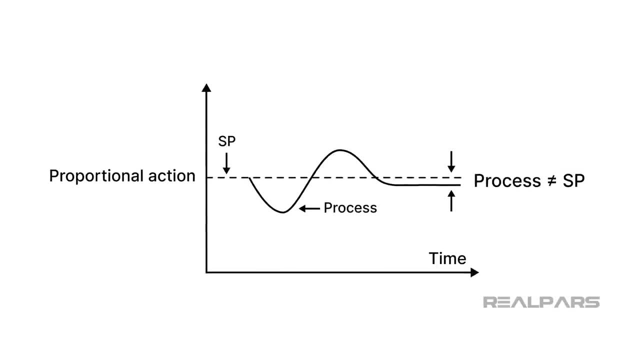 The proportional component applies an effort in proportion to how far the process is away from the set point. Proportional control gets you close to the set point, but not quite there. The integral component applies an effort to return the process to the set point. 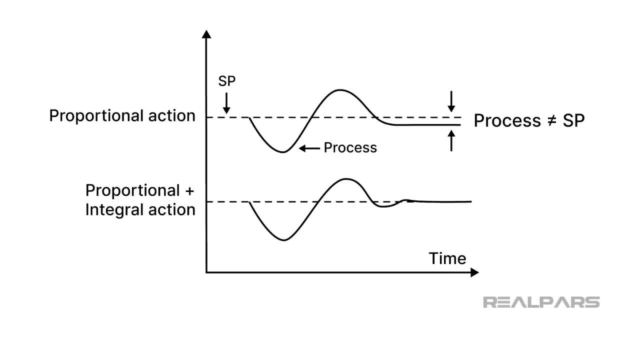 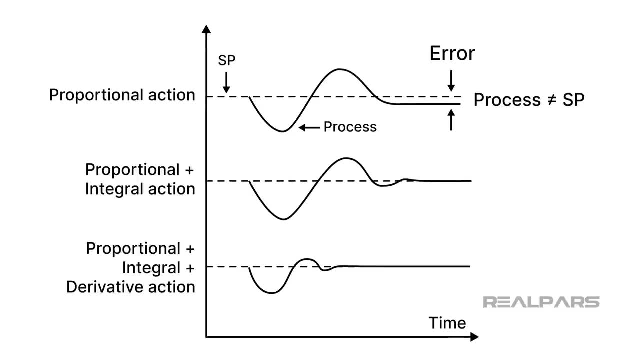 after the proportional control quits, The longer the error exists and the greater the amount, the larger the integral output. The derivative component looks at the speed at which the process is moving away from the set point. Derivative control looks ahead to see what the error will be in the future. 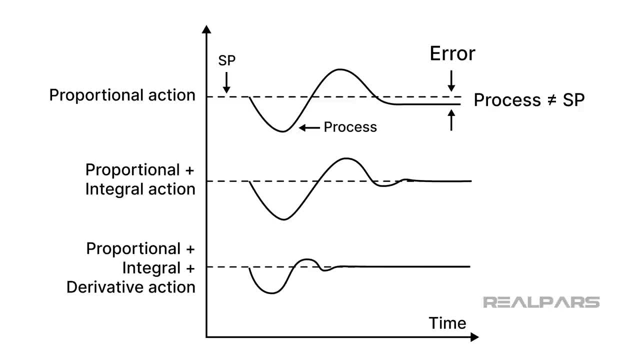 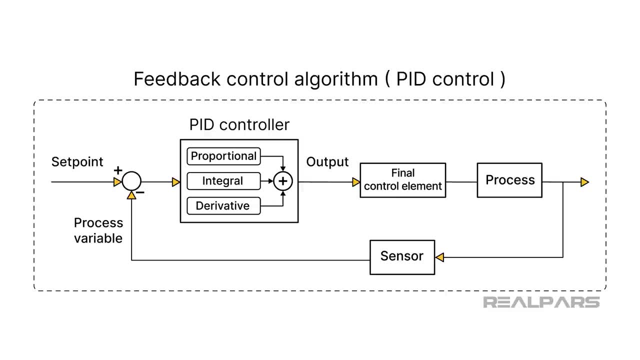 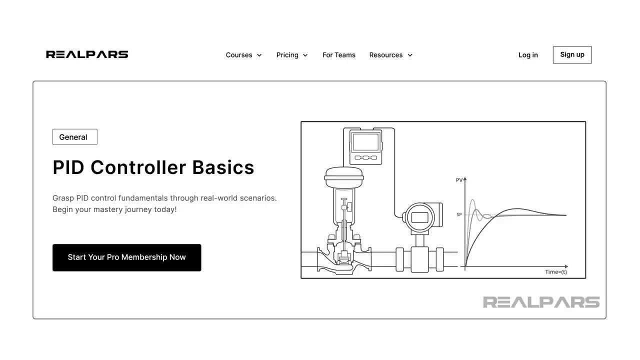 and adjusts the controller output. Each component contributes a unique signal that is added together to create the controller output signal. Alright, that's enough said about PID control. We dive deeper into PID control in our course called PID Controller Basics. You can sign up for this course at realparscom. 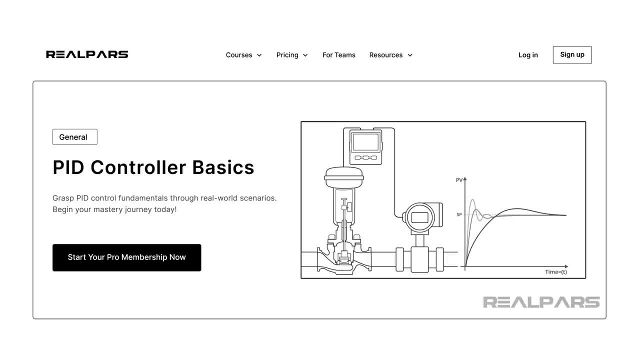 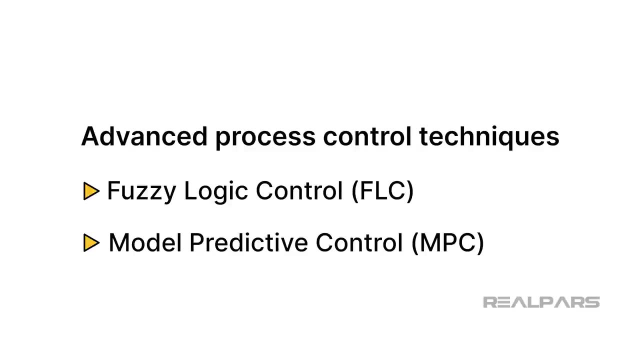 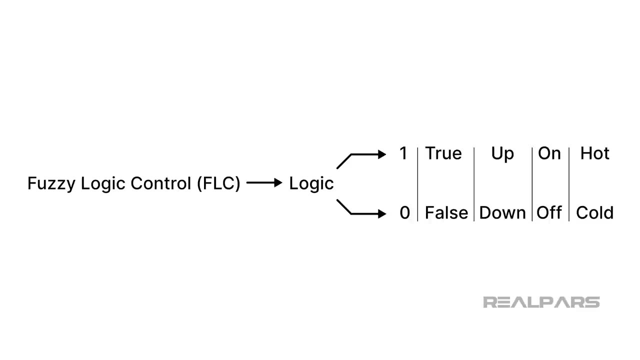 The link is in the video description. Let's move on to advanced process control techniques. We'll start with the first one, the PID control. We'll start with Fuzzy Logic Control or FLC. We've been taught that the binary or logic world has only two possibilities. 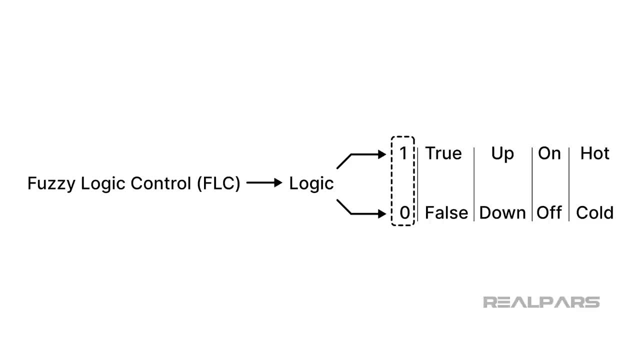 For example, these two possibilities are 1 or a 0, when 1 is true and 0 is false. Stretching the binary concept a bit further, we have lots of linguistic binary pairs such as up or down, on or off. 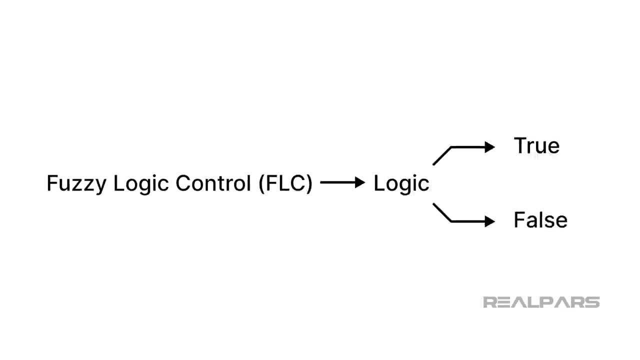 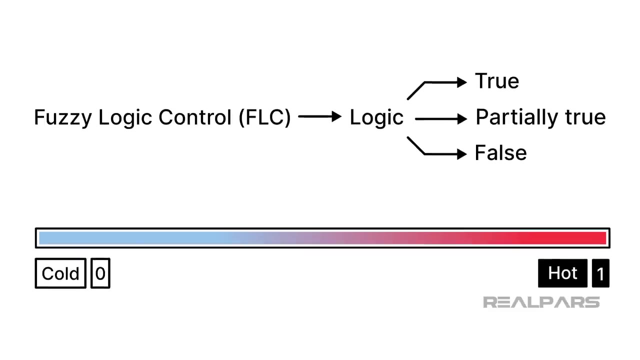 hot or cold. You get the picture. Fuzzy Logic says that there may be more than two possibilities. For example, there might be a partially true in addition to true and false. Based on the Fuzzy Logic concept, we can have lots of values between cold, represented by 0,. 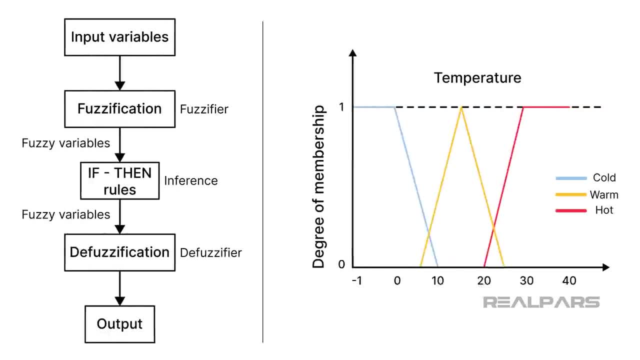 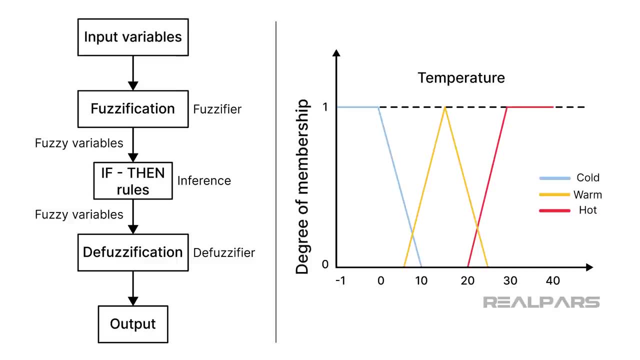 and hot, represented by 1.. Let's look at a very basic example. Fuzzification is the process of converting specific input values into some degree of memory or membership of fuzzy sets, based on how well they fit. Membership functions describe the degree of membership. 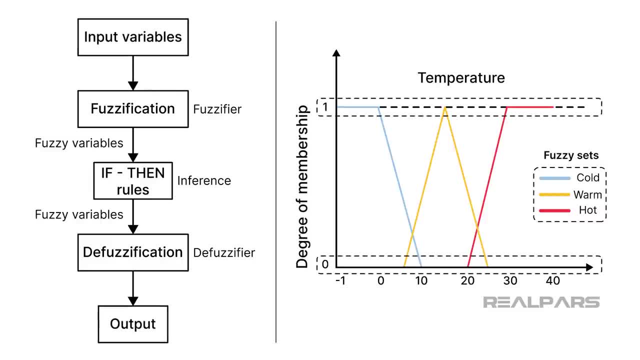 of a particular input or output variable to linguistic variables such as temperature and fan speed. These membership functions can be represented graphically, where each fuzzy set has a degree of membership to a temperature range based on the room temperature. What is a fuzzy set? 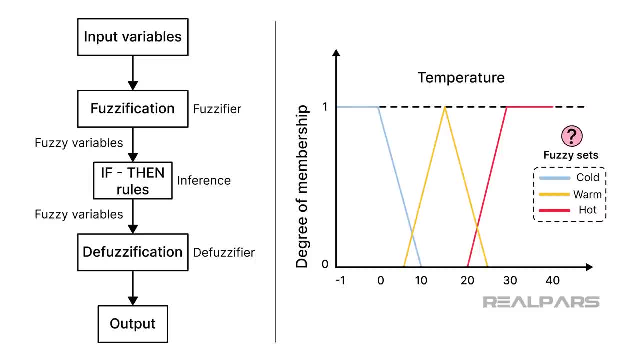 A fuzzy set relates to membership. linguistic variables, for example, a linguistic variable temperature might have fuzzy sets like hot, warm and cold, each with its own membership function. These membership functions help quantify the fuzzy logic involved in making decisions based on linguistic variables rather than precise numerical values. 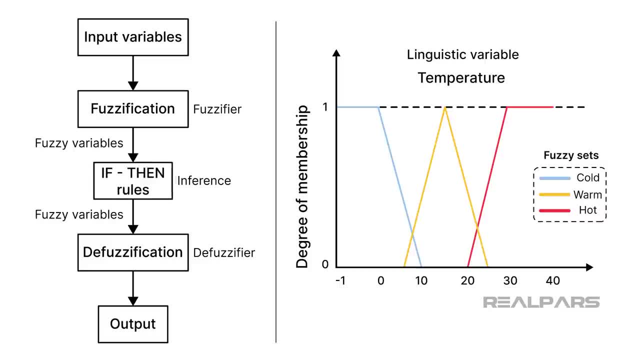 FLC uses a set of if-then rules that express how the input variables relate to the output variable. These rules are based on the input variables and the output variables are based on the input variables. These rules are based on linguistic terms. For example, a fuzzy rule might be: 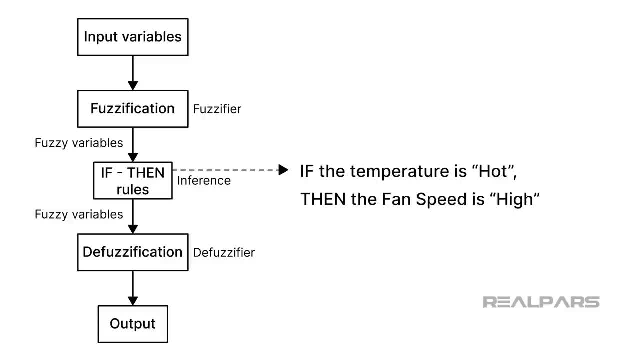 if the temperature is hot, then the fan speed is high. Fuzzy inference assesses how well the input variables match the conditions specified in the fuzzy rules. Finally, defuzzification is the process of converting the fuzzy conclusions into a real-world output value. 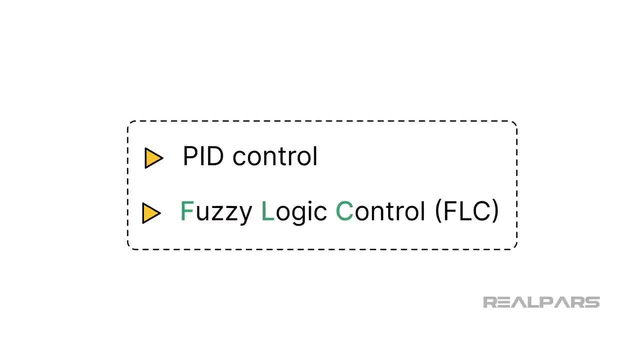 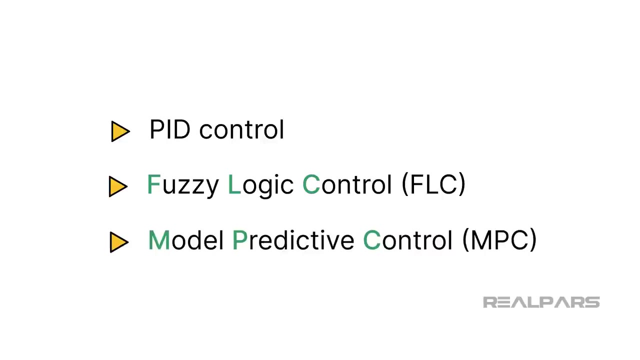 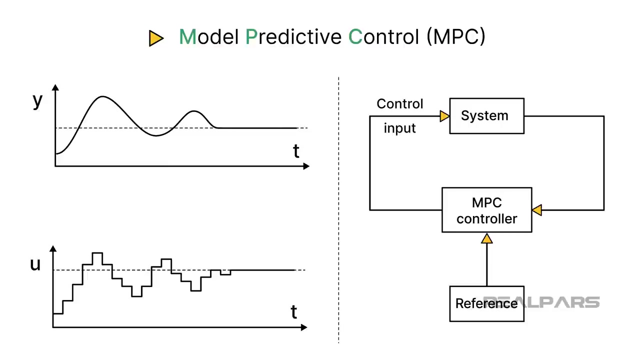 Some vendors have combined PID and fuzzy logic. Some vendors have combined PID and fuzzy logic. The Omega CN74000 series controllers are self-tuned PID controllers with fuzzy logic features. Next up for discussion is Model Predictive Control or MPC. Model Predictive Control, or MPC, is a feedback control technique. 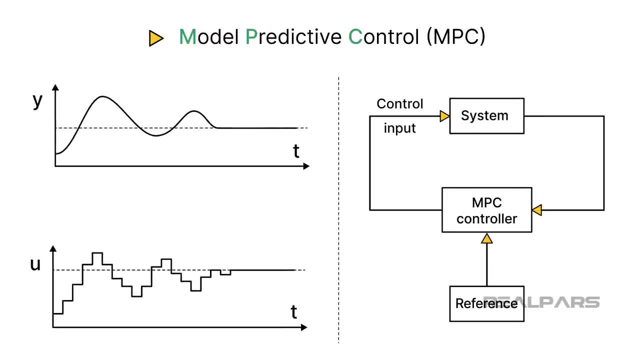 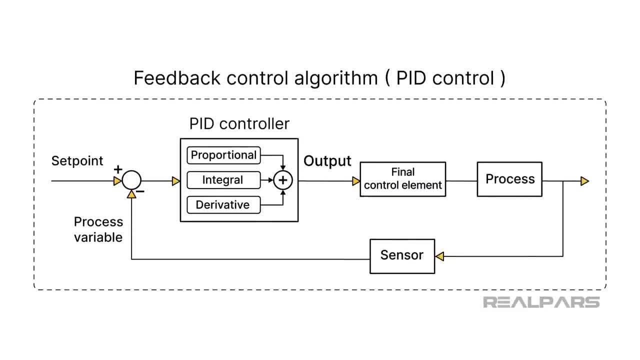 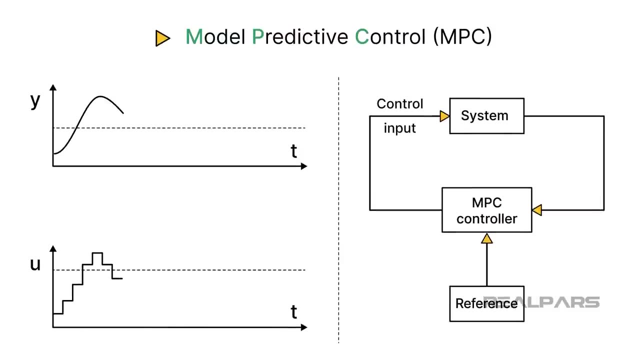 that uses a mathematical model to predict the behavior of the process variable. In contrast to a PID controller that automatically adjusts the control output based on the input data, an MPC controller is a control algorithm that predicts the future behavior of a system based on a mathematical model. 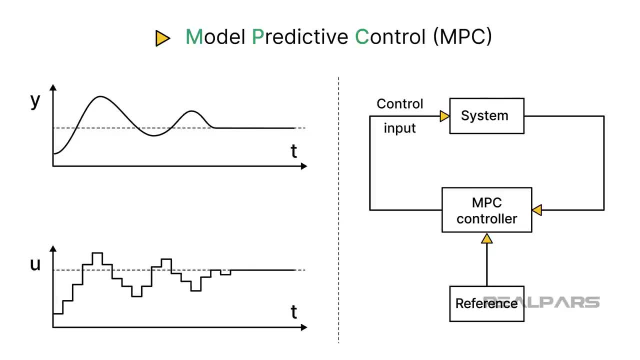 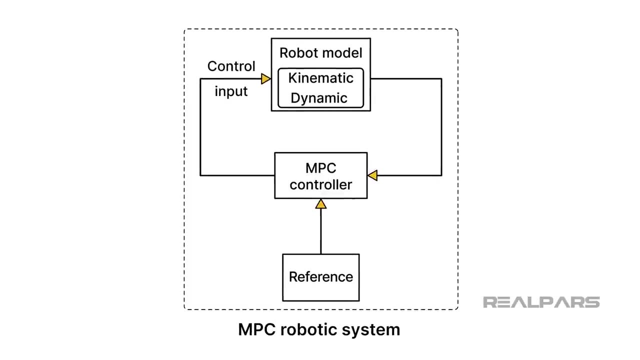 It utilizes this model to optimize and generate control actions. The predictive nature of MPC makes it a powerful and widely used control strategy in many industrial applications. Let's look at a block diagram of MPC for a robotic system. We'll start with the MPC controller components.